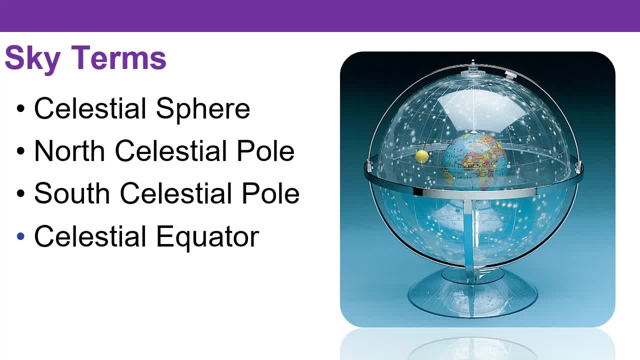 size is actually quite small. It's a big object, but very far away. obviously. Now you'll notice that this yellow sphere is actually on a rod and if you rotate this, the path of this yellow sphere across the sky will represent the path of the sun. It turns out that it can cross the celestial equator. 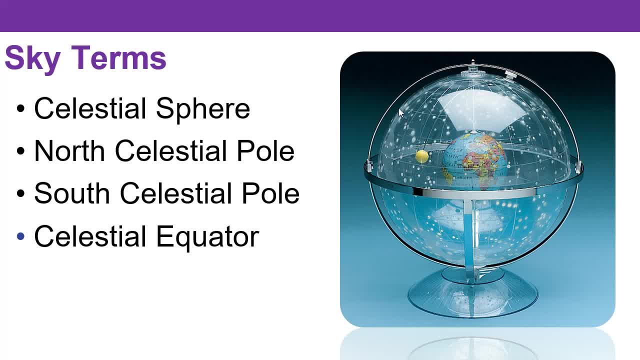 right here. It will rise up and get about this high On the celestial sphere. it will cross again back over there and then come back over here, Go down about this far on the celestial sphere and then back up here again. I talk about it in such great 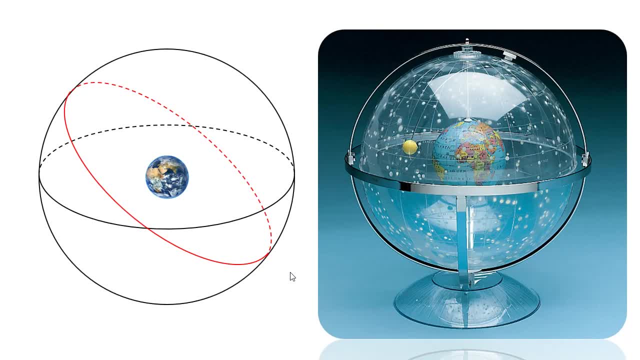 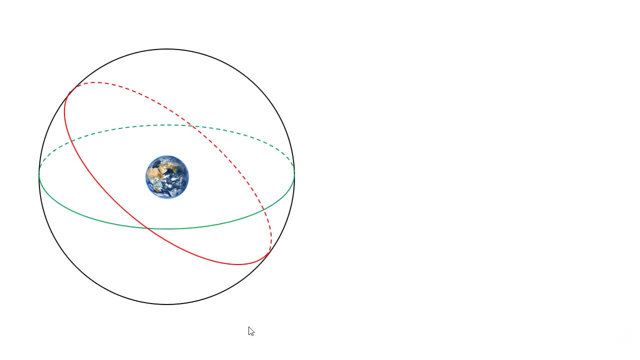 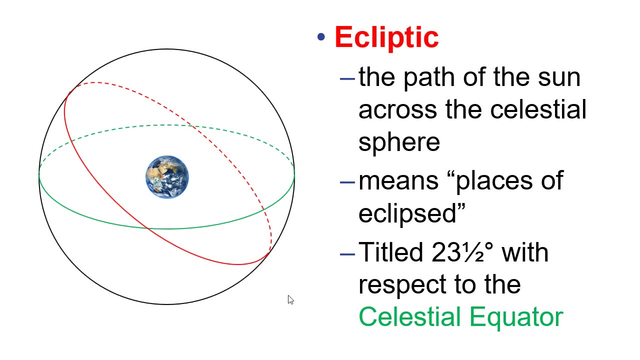 detail, because that's key to the coordinate systems that we use on the celestial sphere. This path of the sun shown in red right here is key to our coordinate systems for stars. This yellow path that we're talking about here is called the ecliptic. Some things that you need to know about the ecliptic is. number one is the path of. 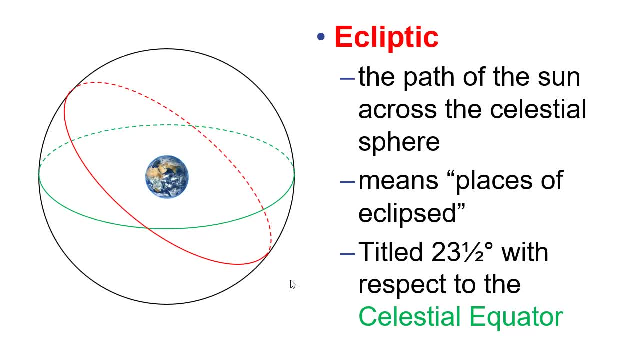 the sun across the celestial sphere. So the sun moves through the stars. I mean, you really can't see that, because in the daytime the sun is, you know, hiding all the constellations from us. But it turns out that it's just moving in front of the 12 zodiac constellations throughout the year. 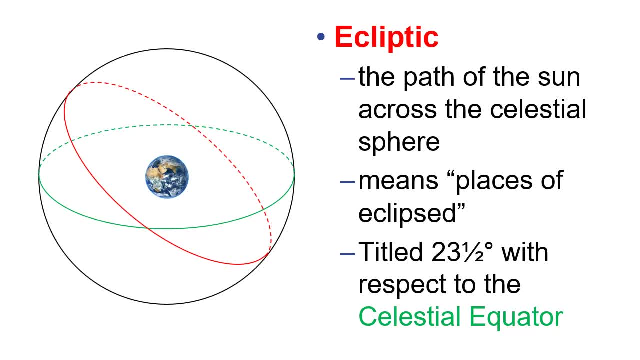 Just creeping across there. Now it turns out that the sun is not actually moving. It's us that's moving, But from our perspective, it looks like the sun is rising and setting. It looks like it's going through constellations. So that's the perspective we're going to talk about. So from our perspective, 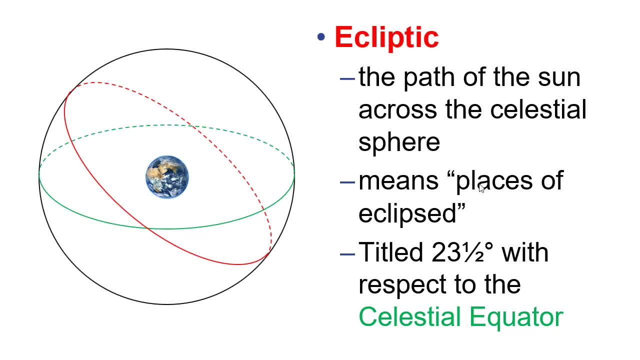 it looks like the sun is going across the celestial sphere and this red curve that you see here is tilted a little bit with respect to the green one, which is the celestial equator. So this angle right here, 23 and a half degrees between the celestial equator and the ecliptic. 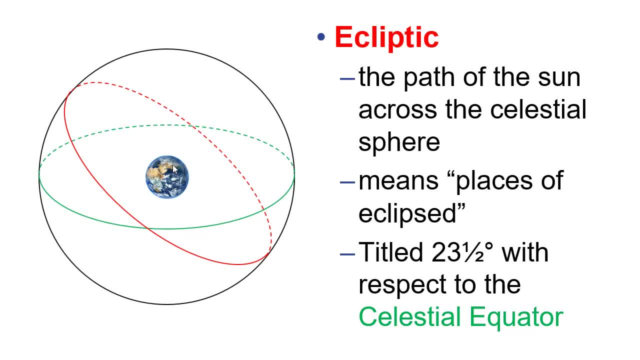 The reason it's 23 and a half degrees is because the earth's axis is tilted 23 and a half degrees. It's a little typo right here. This second bullet should say: ecliptic means places of eclipses. So our ancestors noticed that the solar and lunar eclipses. 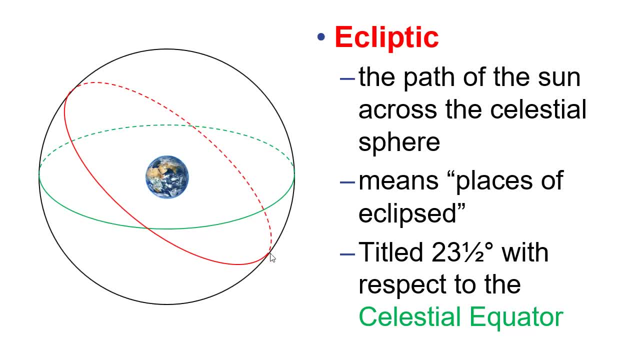 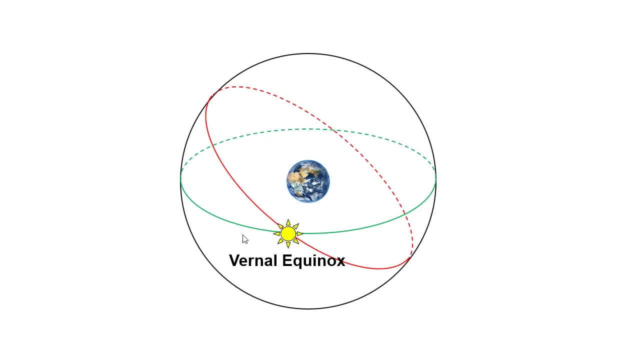 would always occur in these dozen or so constellations around the ecliptic. They would always occur in the same place. So this is a collection of constellations. Now there are two intersection points between this red thing and the green thing, And by red I mean ecliptic and celestial equator. 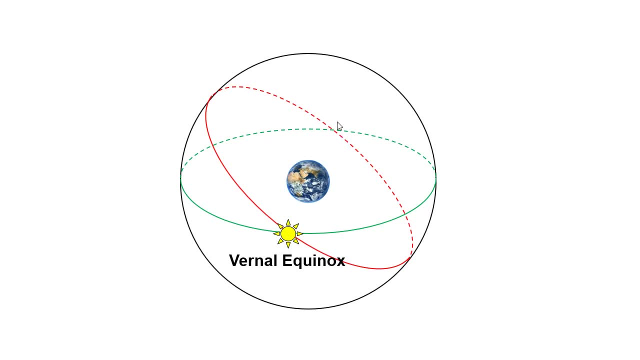 So there's an intersection point here and an intersection point over there. This is called the vernal equinox. It turns out when the sun is right there. it takes place on the same day of the year roughly every year, And vernal means spring and equinox means equal days, equal nights. 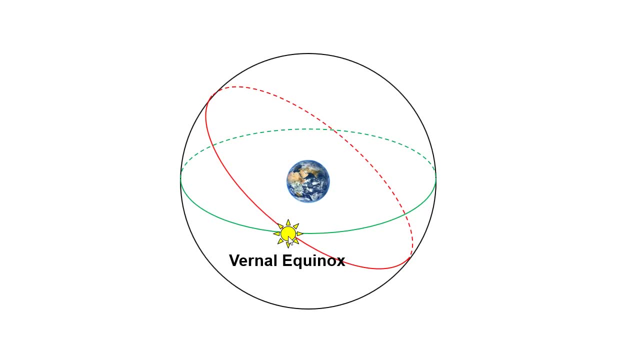 In other words, on this day of the year there is 12 hours of daylight, roughly, and 12 hours of darkness, So equal nights. I guess you can think of it in that way. anyway, This is the first day of spring. As the year goes along, the sun will rise up on the celestial. 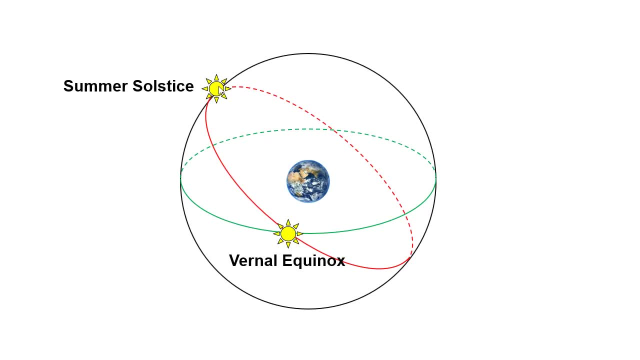 sphere, going across the ecliptic up here Until the sun gets to its stopping position here. So the sun rises and then it reaches a stopping position and starts to come back down And SOL stands for sun and then the last of this is stop. 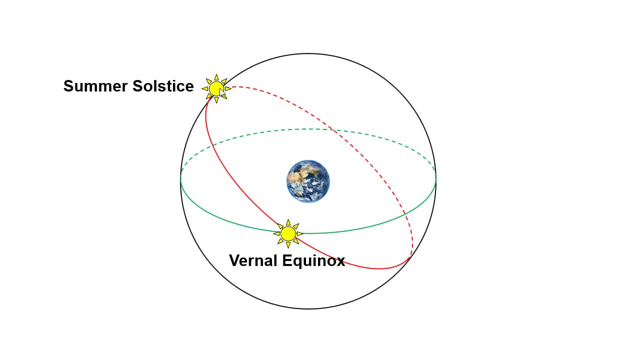 So the sun stops when it gets right up to the top, And it turns out that during that time of year, around June 22nd- in the northern hemisphere at least, that's our summer time- The other intersection point occurs on the first day of fall. I think it's around September 22nd. 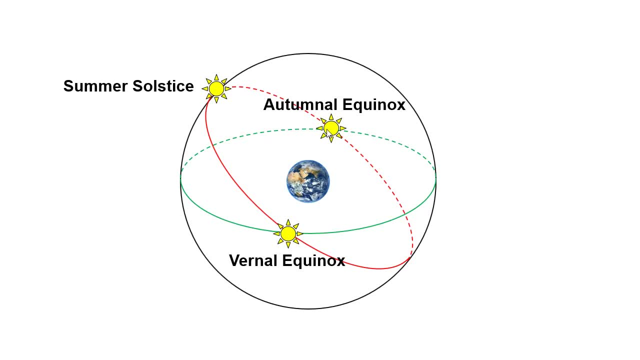 The first day of fall, And on this day you also have 12 hours of daylight and 12 hours of darkness. Now, on the summer solstice, it's not that way. You have more than 12 hours of daylight and less than 12 hours of darkness, And I bet you know what this point down here is called. 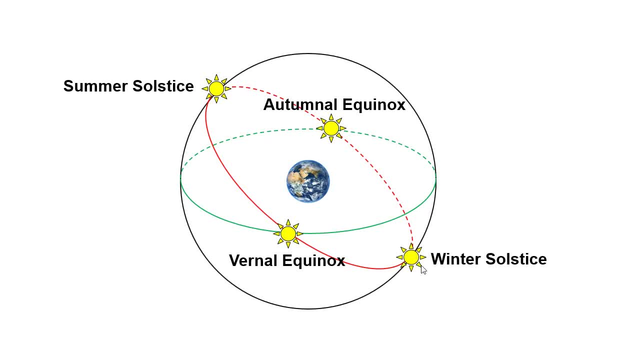 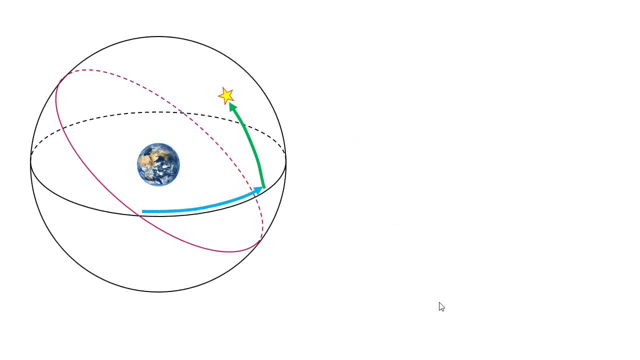 That is the winter solstice, and here we have more hours of darkness and then daylight, and also in the northern hemisphere the sunlight is more at an angle here, so we don't get the direct sunlight and therefore it's cooler during this time of year. So this is what really causes seasons. is that tilt of the earth's axis? That's really what causes. 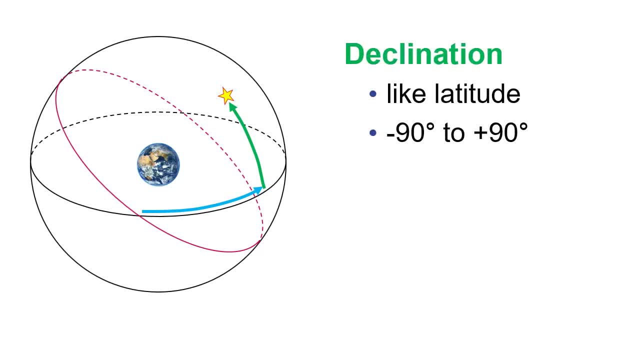 the seasons on the earth. We mentioned this in class a little bit- that this coordinate system that is very similar to latitude, is measured above and below this celestial equator from zero degrees on the celestial equator to positive 90 up here, negative 90 there. You'll be using that in your laboratory exercises early on this semester. 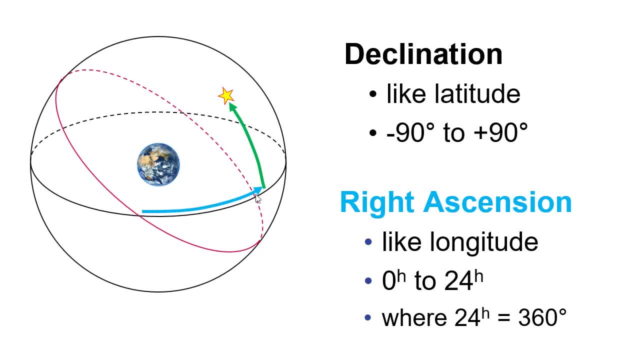 And the blue arrow is measured around the celestial equator. along the celestial equator like longitude, and notice that the place that you start is the bernal equinox. That's the part we didn't get to in class last time. So instead of starting at greenwich, england, like you would do for 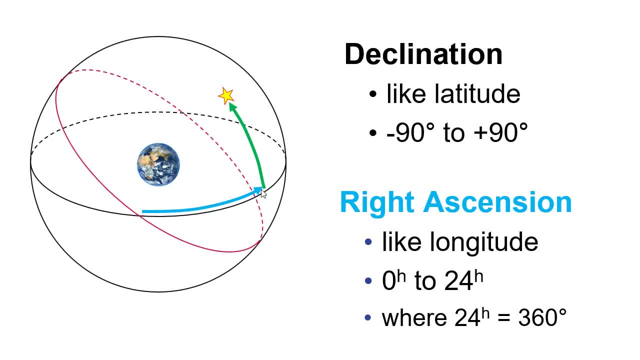 longitude you actually start at the bernal equinox measure around the other thing. that's different and you might remember, for longitude we went from zero degrees to 180 east, zero degrees to 180 west. but in the case of right ascension, astronomers have introduced a new angular measurement. It's 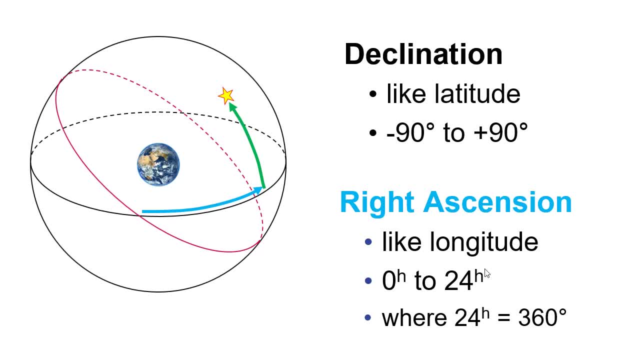 zero superscript h up to 24 superscript h, and so it looks like it's an hour which is a unit of time, but really it's an hour unit of angle, where 24 hours of angle corresponds to 360 degrees. It's kind of an odd thing if you. 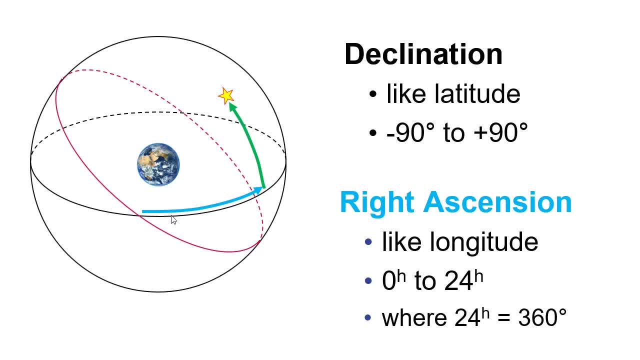 think about it. but suppose you start here and you went all the way around here that would correspond to 360 degrees, but it also would correspond to 24 hours in our new unit of angular measurement called hours. So declination measured in degrees, right ascension measured in hours. 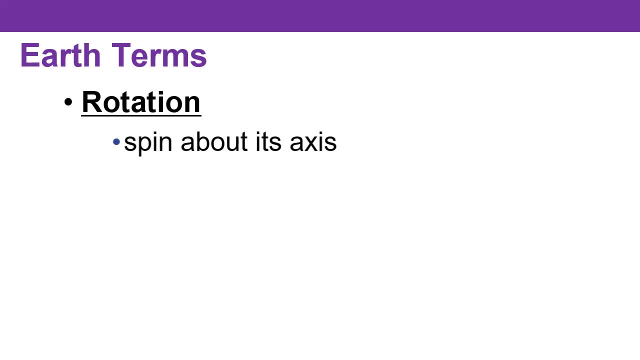 Some more earth terms. It's important that we distinguish between two key things that deal with spinning and circular motion. The two terms here are rotation and orbit. We want to make sure we keep those separate as we begin to talk about stars, planets and galaxies this semester. 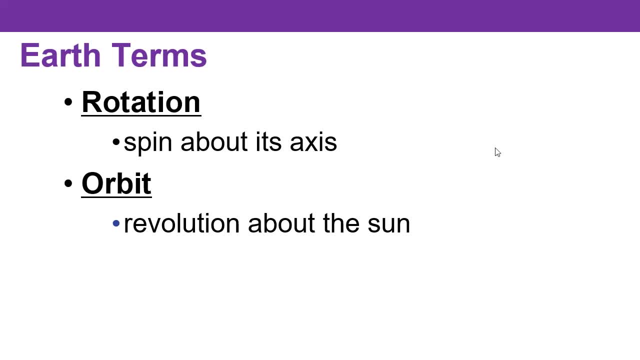 A spinning about an axis, like the earth spinning about its axis once every 24 hours- that's going to be referred to as rotation- and then As it moves around the sun in its orbit, we can call that revolution about the sun. That happens 365 and a quarter rotations days per year. 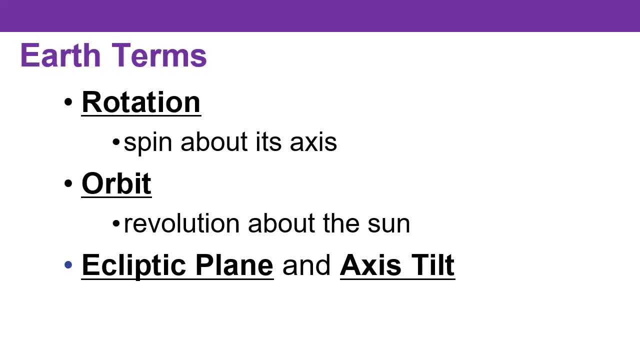 Now there is another way to look at this ecliptic and that is in terms of a plane. It really defined a plane in our previous diagram, but I want to show you in this next sketch a couple of things. We want to focus on the ecliptic plane and the axis tilt of the earth. 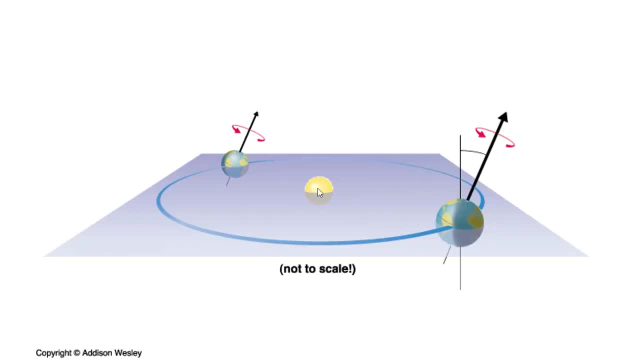 Here is the drawing coming up next. This is not a celestial sphere model, but instead more of a somewhat more realistic model. I like how it says not to scale, because the sun is obviously much bigger than that. The size of the earth is magnified so that you can see this tilt of the earth's axis. 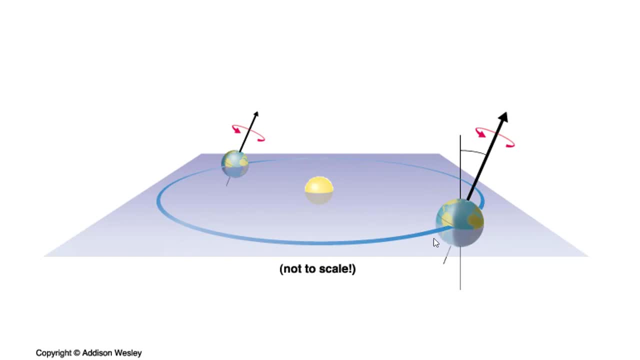 This circle. here is the earth. This is the earth's orbit and it defines the ecliptic plane. This blue thing is called the ecliptic plane. The red line we saw in the celestial sphere is called just the ecliptic. 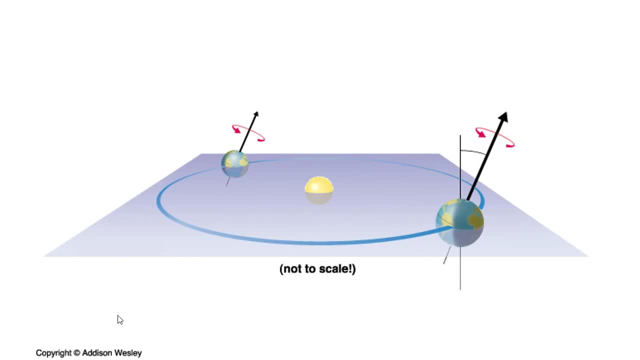 but the plane that exists actually out in space is called the ecliptic plane. The other thing that we notice is that the axis of the earth is tilted. You probably already knew that already, but I want you to know that it is pointing to a relatively bright star called Polaris. 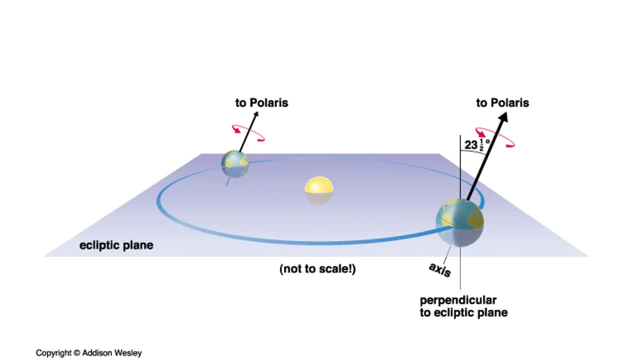 Polaris is also known as the North Star. so Polaris and the North Star, they're the same thing. You'll notice that during this season right here, I think this might be the Revernal Equinox It's pointing up and to the right to Polaris. 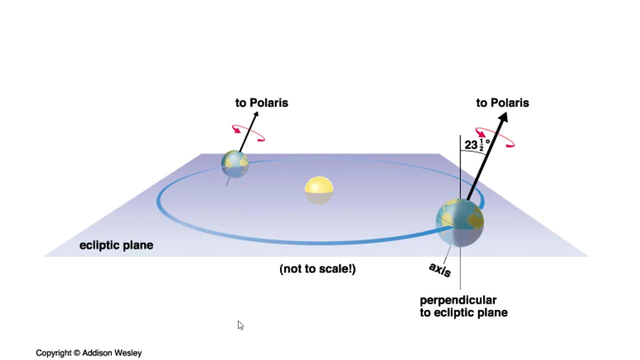 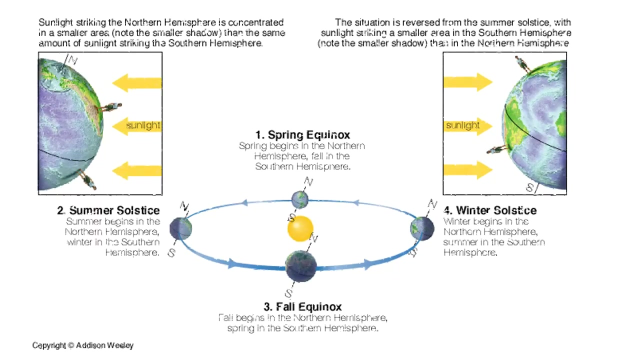 We notice the same kind of thing out here for the Autumnal Equinox. This 23.5 degrees is the cause of those red and green circles shown before Being at a tilt of 23.5 degrees. One thing you should also know as we get into some multiple-choice questions. 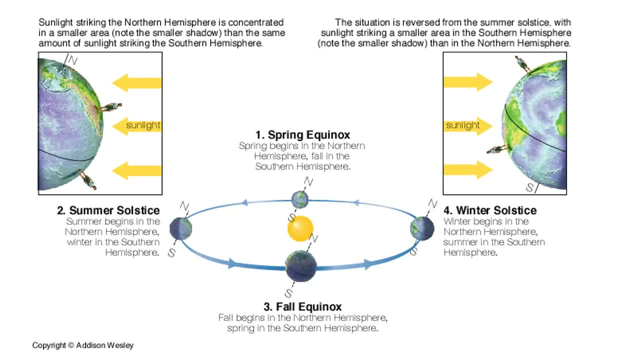 as it tries to demonstrate here. the seasons are caused by the tilt of the Earth's axis. It's not that the Sun and the Earth are any closer in the summertime, like this right here. It's just that the part where we're at is tilted more toward the Sun in the summertime and tilted